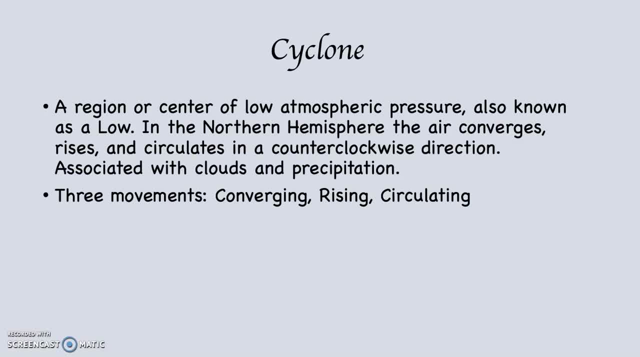 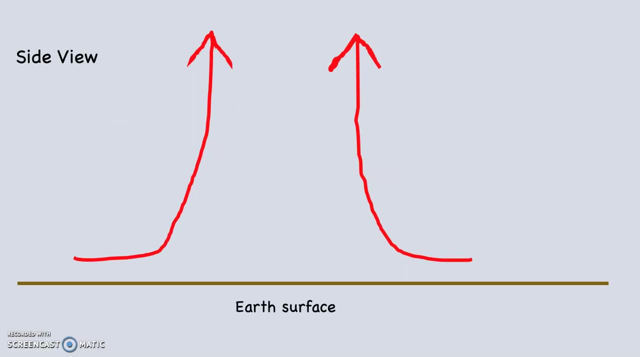 Keep in mind. there are three movements. This is critical that you keep the movements in mind: Converging, rising and circulating air. Let's take a look. I built this little diagram for you. This is a side view. Imagine that you're looking out across the landscape and you can see the movement of the air. 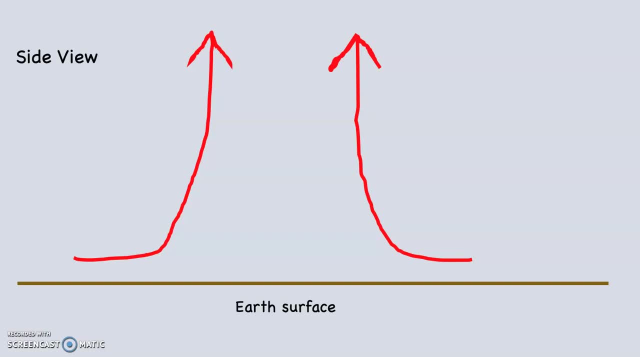 Imagine that you're looking out across the landscape and you can see the movement of the air. you cannot, but if you could see the movement of the air. the red arrows are representing the movement of the air in a low-pressure system, which is the air is going to converge and rise. 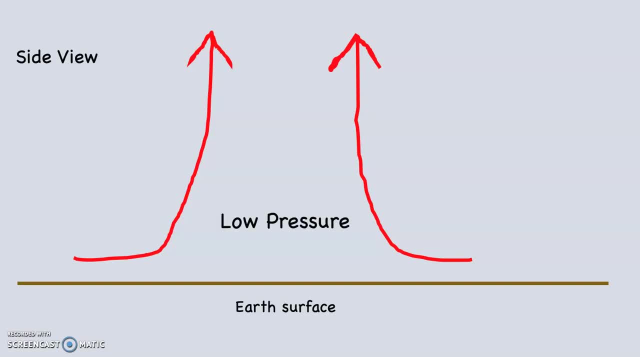 When you have converging rising air. this is what creates a low-pressure system. Well, it may not be the thing that creates it, but this is the result of it. Now, if you look, you can see that indeed. 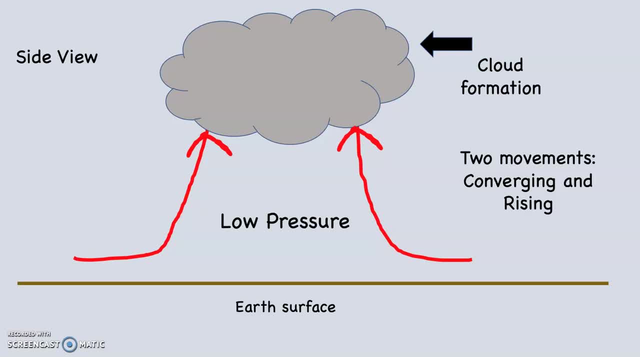 there are clouds forming because low-pressure systems, cyclonic systems, are associated with clouds and notice. there are three movements. So far we have two of them. We have the converging and rising characteristics of low-pressure. but there is a third movement, which is circulation. 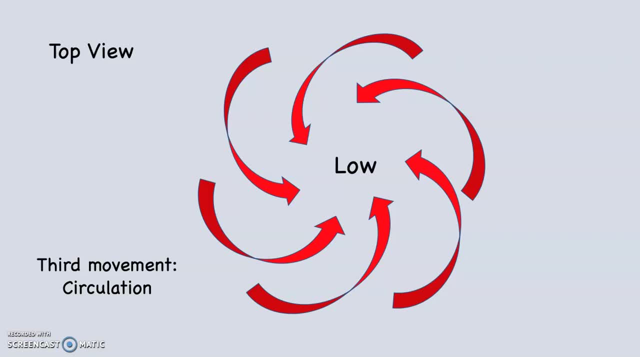 If you were up in space watching a low-pressure system move in the northern hemisphere, the circulation would look like this, which is counterclockwise and in Notice. as you're looking at those arrowheads, the arrowheads are pointing towards. 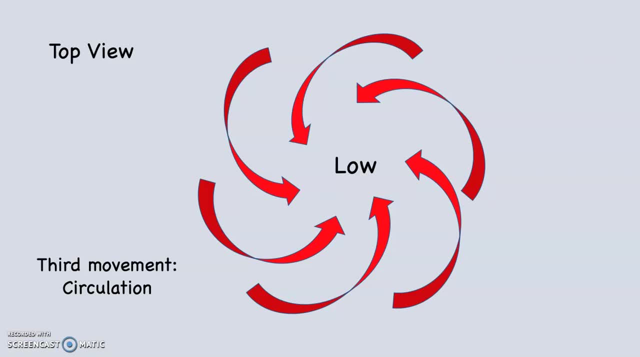 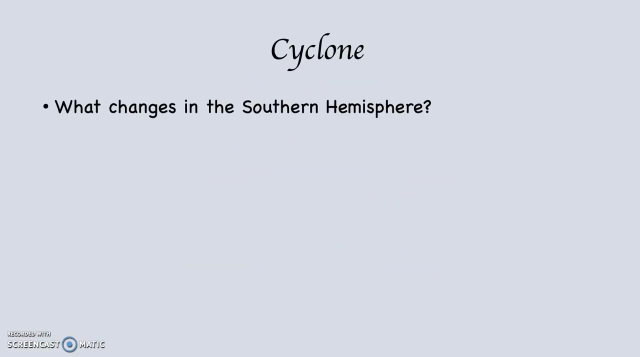 the low. So it's not just making a circle around the low, it's counterclockwise and spiraling inwards. Okay, so, converging, rising, circulating, Good. Of course I did say the northern hemisphere. What changes in the southern hemisphere? Well, there are three movements. 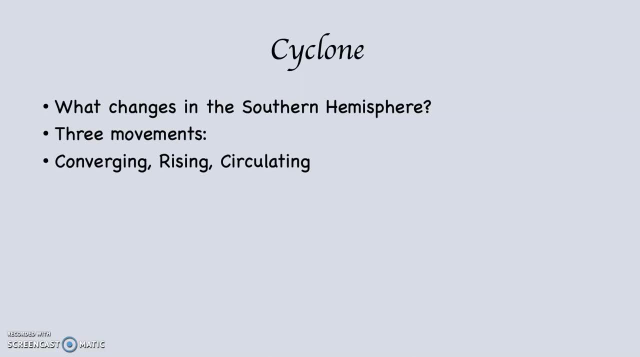 Right, There's converging, rising and circulating. Converging and rising are always part of low-pressure systems, cyclonic systems. So there's never going to be a moment that converging and rising air are not part of low-pressure systems. What changes in the southern hemisphere is circulation? 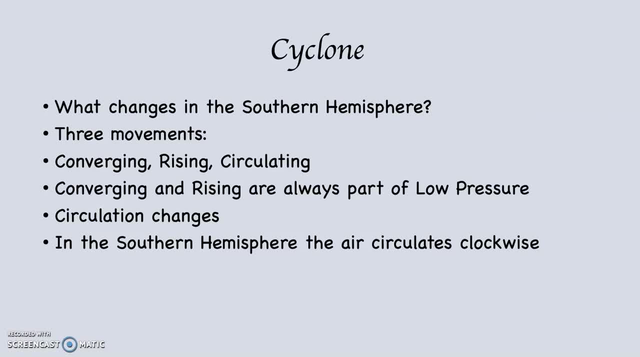 In the southern hemisphere the air circulates clockwise and in Make sure you know those things. Make sure you know converging and rising is always part of a low-pressure or cyclonic system, but that the circulation changes, It's always going to go inwards with low pressure. 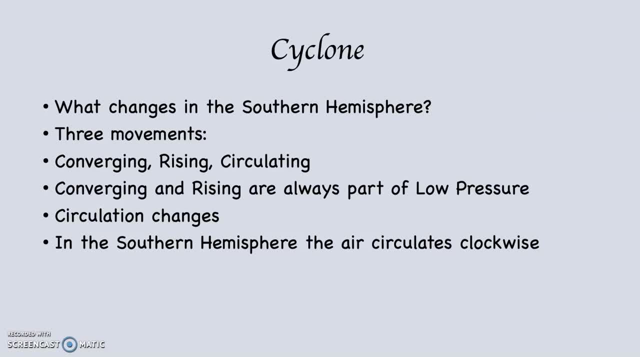 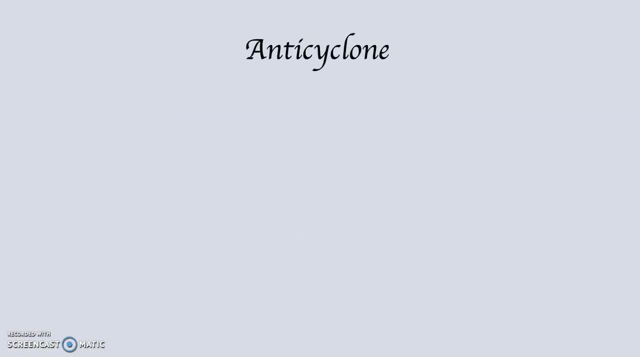 but in the northern hemisphere that will be counterclockwise and inwards, and in the southern hemisphere that will be clockwise and inwards. The second type of system is called an anticyclone or anticyclonic system. This is a region or center. 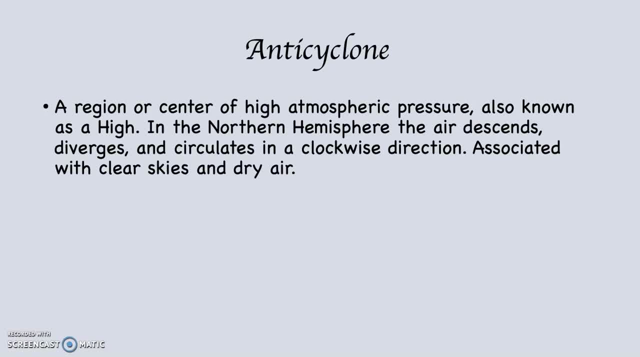 of high atmospheric pressure, also known as a high In the northern hemisphere. the air descends, which means it subsides, it comes down, diverges, which means it pulls away from the center and it circulates in a clockwise direction. High-pressure systems, anticyclonic systems. 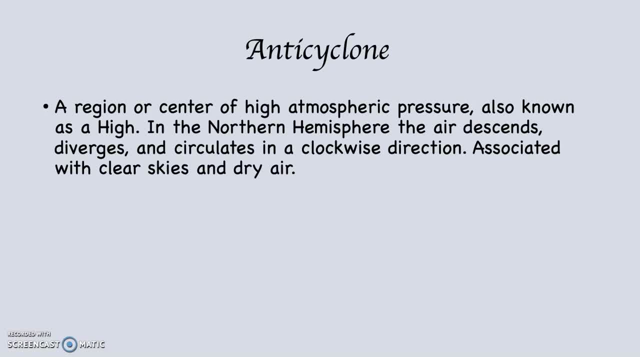 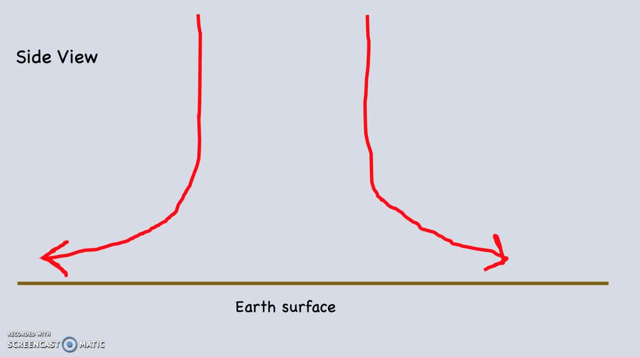 anticyclone, high-pressure are synonyms, are associated with clear skies and dry air. Again, keep in mind, there's three movements: Descending, diverging and circulating. Take a look at this diagram Again. you're looking across the surface of the planet and, as you look across the surface of 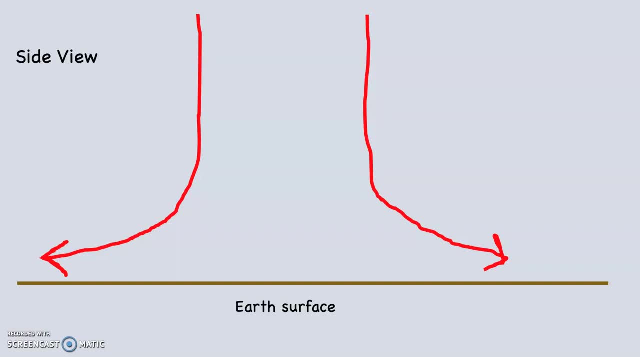 the planet. if you were able to see the movement of the air represented by the red arrows, what you would see would be the air would be descending from aloft and as it came down towards the surface of the planet, the air would be diverging- exactly what you see there. That is a hallmark of high. 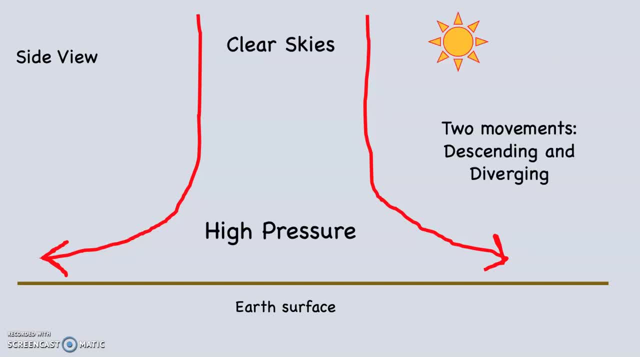 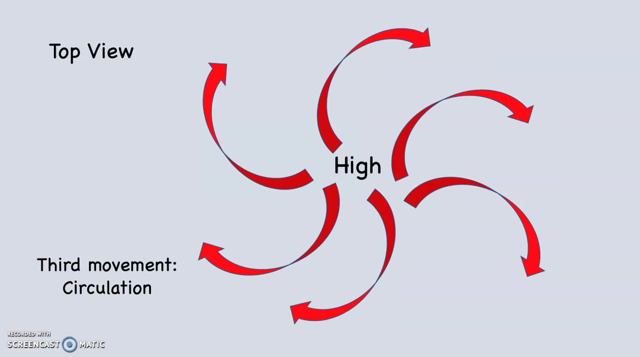 pressure, And of course, high pressure is associated with clear skies. You can see the sun there, But notice, we only have two of the movements so far: Descending and diverging. The third one is Circulation. Again, if you were up in space and you were somehow able to see the movement of the air around, 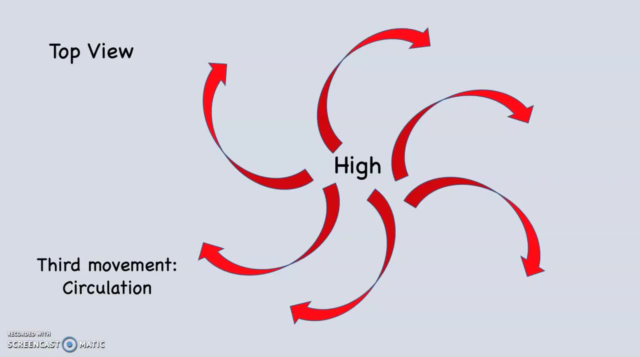 the high pressure system. what you would see would be this: The air would be circulating in the northern hemisphere clockwise and out. Now look at those arrowheads. They are not pointing back at the high, They are pointing away from the high. So the movement in the northern hemisphere is